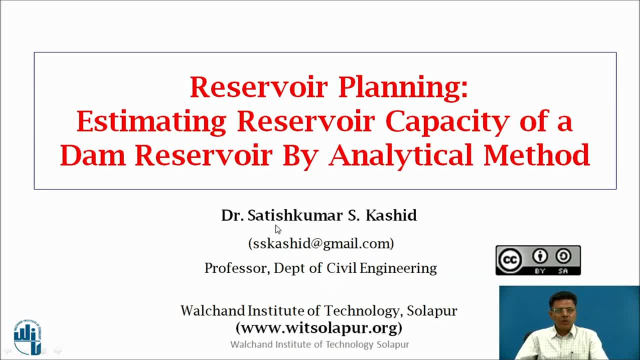 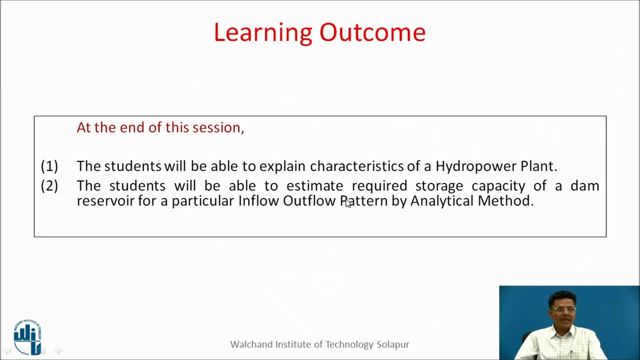 Hello, I am Dr Satish Kumar Kashyad, Walchand Institute of Technology, Solapur, presenting a topic: Reservoir Planning: Estimating Reservoir Capacity of a Dam Reservoir by Analytical Method. Learning outcomes of this session. At end of this session, the students will be able: 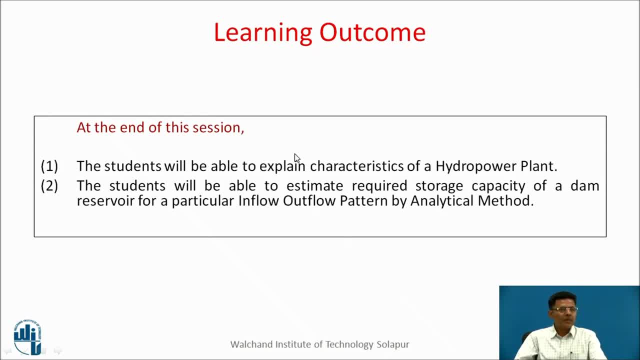 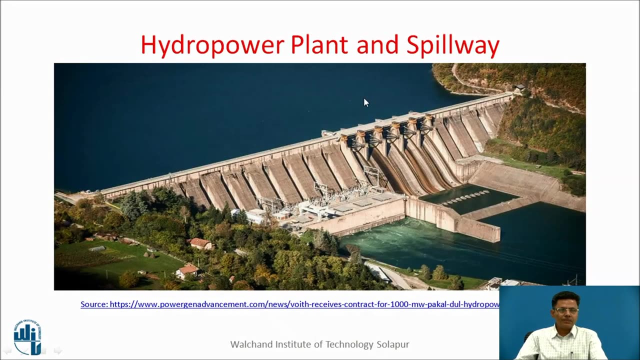 to explain the characteristics of a hydropower plant and the students will be able to estimate required storage capacity of a dam and its reservoir for a particular inflow pattern by analytical method. One simple example we will take Now. just observe: this is a hydropower. 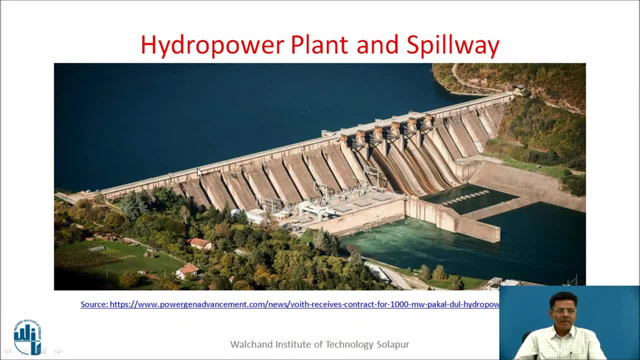 plant and spillway. So this is a barrier in form of a dam which is constructed. This is a spillway portion of a dam or overflow portion of a dam. We observe the gates here, the tenor gates. These are provided here Whenever excess water comes in the reservoir and we need to release. 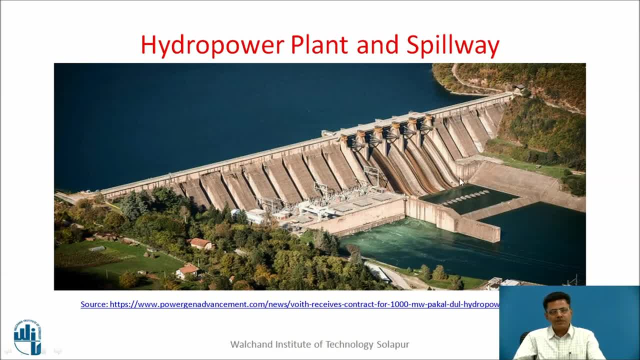 it. we open these gates and allow this water to flow. When we want to generate hydroelectricity, we allow the water to pass through the hydropower generation stations, the turbines which are provided here. So whenever the reservoir is full and inflow is more than required, 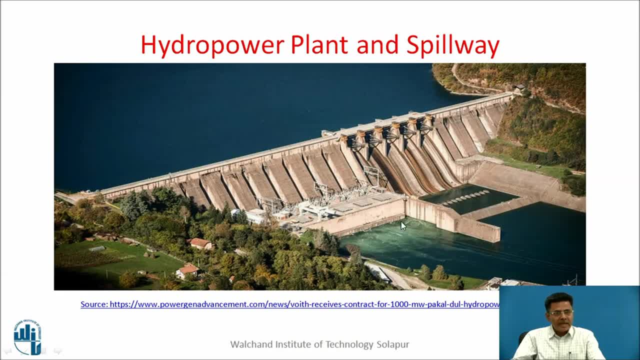 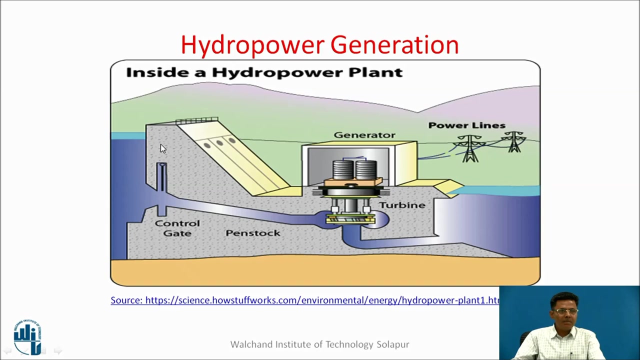 then hydropower generation will be there as well, as there will be spill over the spillway, But when inflow was lesser than the required outflow, in that case, while we will be using water which is stored in the reservoir- Just see, this is the dam, this is the reservoir. form and there is a control gate and these are the että and this is the viendo. then, lower in the reservoir, People in reservoir can also use all ponds here and here, from sides, Here. there you see the الدucto. Here is another section. the other is prepared. 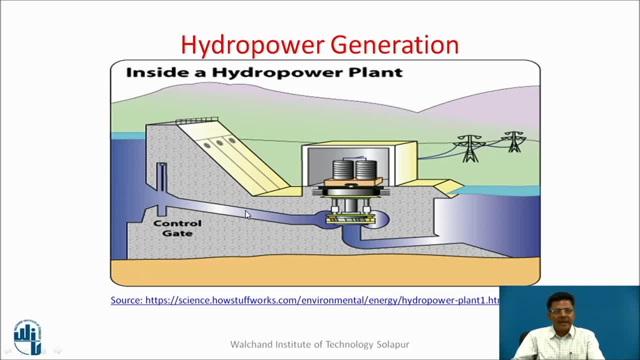 glue here. here this is the control gate which is provided here. These are the pincels. in rain stock, water enters, passes to this turbine, rotates the turbine, the vertical shaft, rotates this particular coil in generator. electricity is generated and sent to the grid. 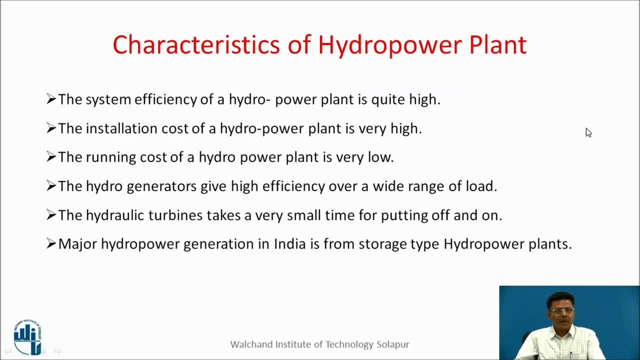 So this is the hydropower generation. Now let us discuss some important characteristics of hydropower plant. The system efficiency of hydropower plant is quite high. The installation cost of hydropower plant is very high. The running cost of hydropower plant is very low. 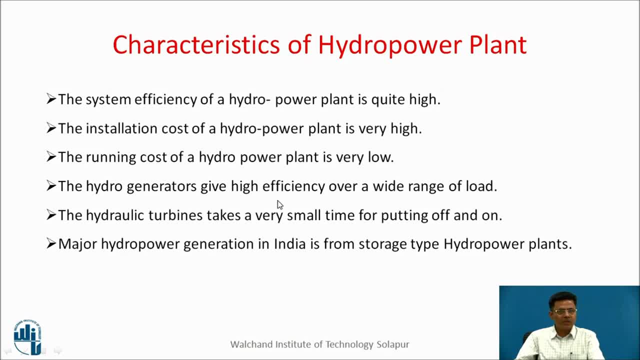 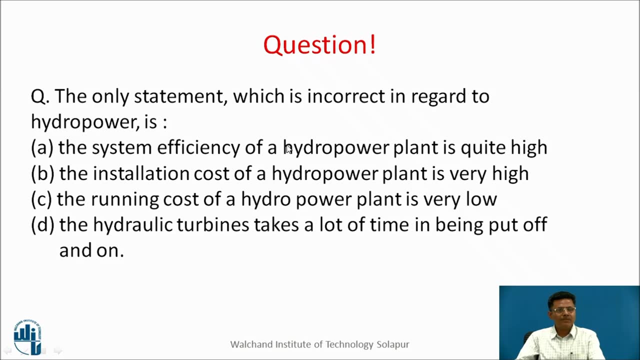 The hydro generators give high efficiency over wide range of a load. The hydraulic turbines take a very small time for putting off and on And the major hydropower generation in India is from storage type of hydropower plants. A small question. The only statement which is incorrect in regard to hydropower is the system efficiency of 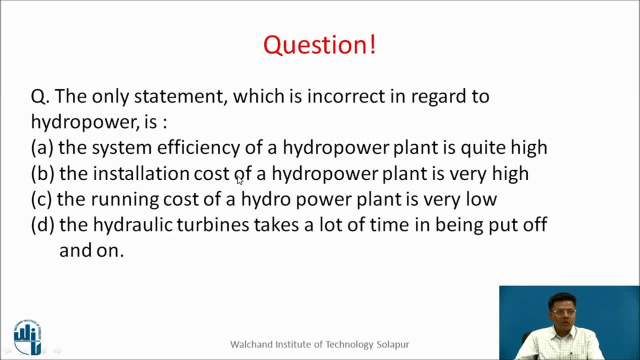 hydropower plant is quite high. The installation cost of hydropower plant is very high. The running cost of hydropower plant is very low. The hydro hydraulic turbines take a lot of time in being put off and on. Obviously answer. the incorrect statement is: the hydropower turbines takes a lot of time. 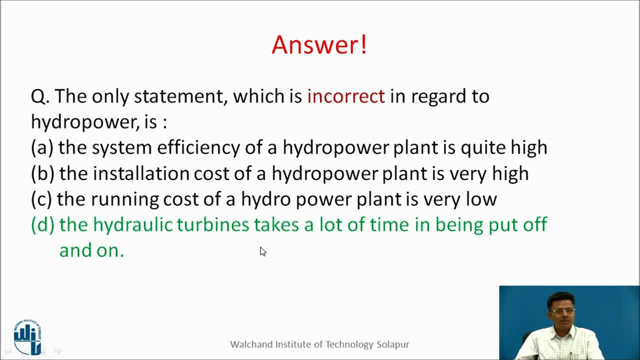 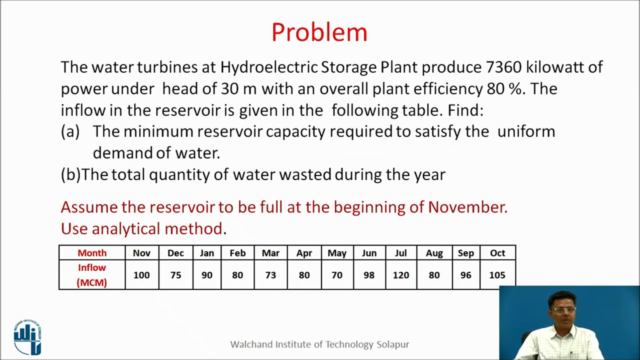 in being put off and on. This is not true, But rather this is applicable to thermal plants, which take a lot of time for putting on and off. Hydropower plants can be made off and on in relatively very short durations. Let us take one problem. 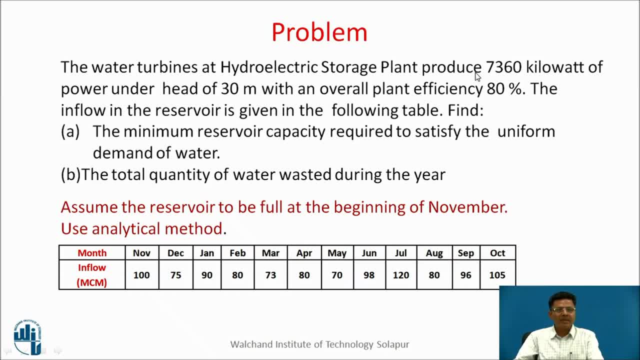 The water turbines at hydroelectric store plant produce 7360 kW of power under head of 30 m, with an overall plant efficiency of 100 kW. The water turbines at hydroelectric store plant produce 7360 kW of power under head of 30 m, with an overall plant efficiency of 100 kW. 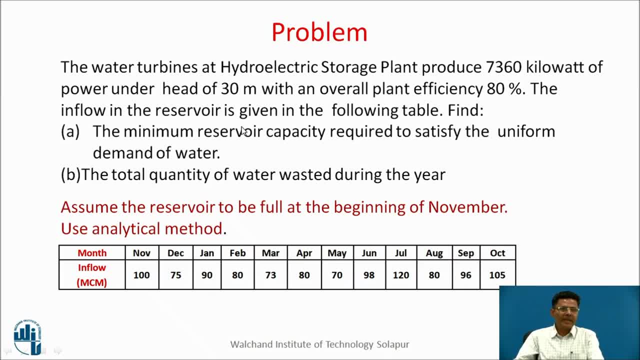 The 160 EACH. it says. The inflow in reservoir is given in the following table: The minimum reservoirs capacity required to satisfy the uniform demand of water. The minimum reservoirs capacity you require to satisfy the uniform demand of water. The minimum reservoirs capacity you require to satisfy the uniform demand of water. 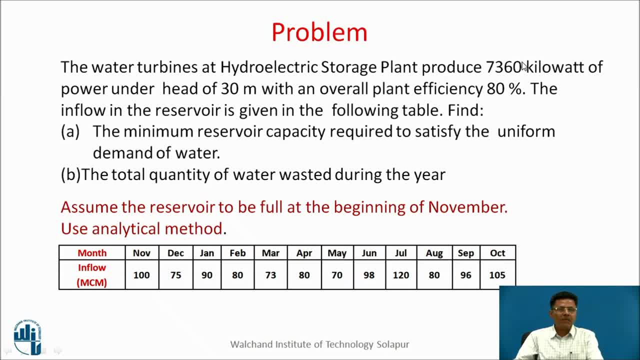 The uniform demand will be decided by the water discharge required to produce 7360kW. We are also asked to find out the total quantity of water wasted during the year. Assume the reservoir to 돼 full at beginning of November and you are asked to use the analytical method. so these are the months. 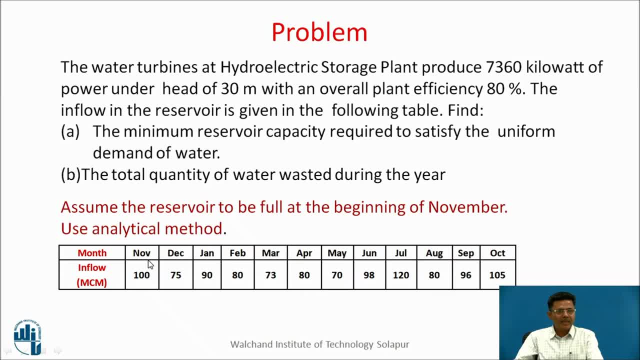 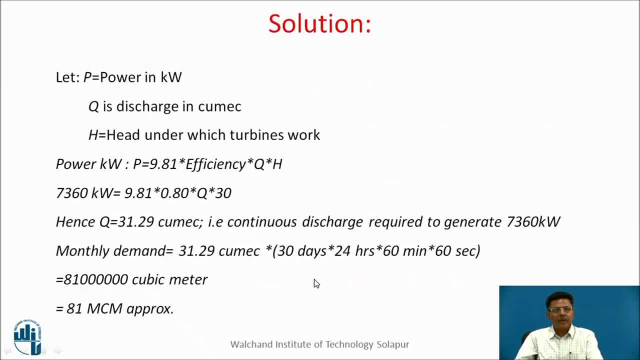 over a year. so at start of November we are assuming reservoir full and then monthly inflows in million cubic meters are given in this way. okay, now let us calculate what is the discharge required to generate 7360 kilowatt continuously. let p be the power in kilowatts, let q is the discharge in. 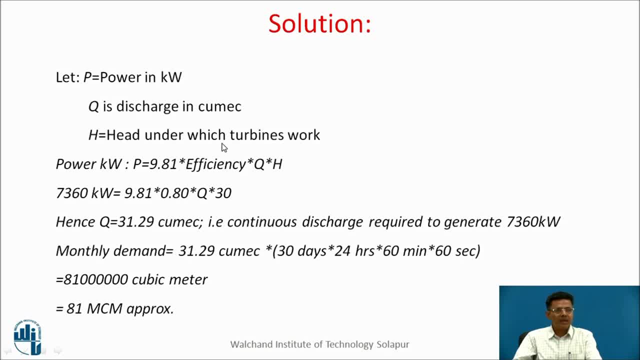 cubic, let h is head under which the turbine work. so power in kilowatt- this is the equation- is 9.81 into efficiency, into discharge, q in cubic, into head h in meter. so putting this value 7360, efficiency 80 percent and head 30 meter, we can find out q. so to generate continuously this 7360 kilowatt we need 31.29. 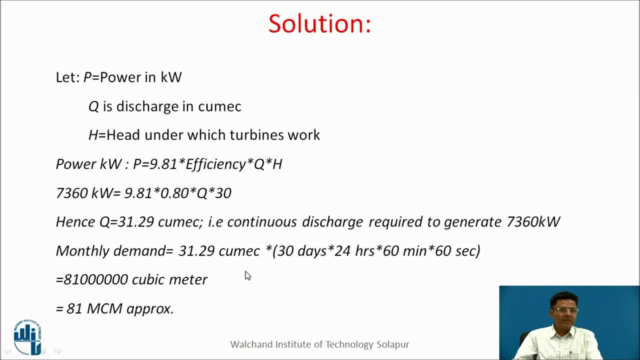 meter cube per second as a continuous discharge. so we multiply it by 30 days, 24 hours, into 60 minutes and 60 seconds. it means this term, this bracket, will give you number of seconds and this is meter cube per seconds. so answer is it 1 million cubic meter approximately. so we need 81 million cubic meter of water. 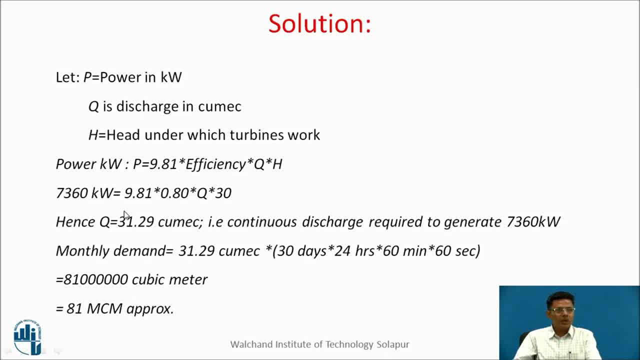 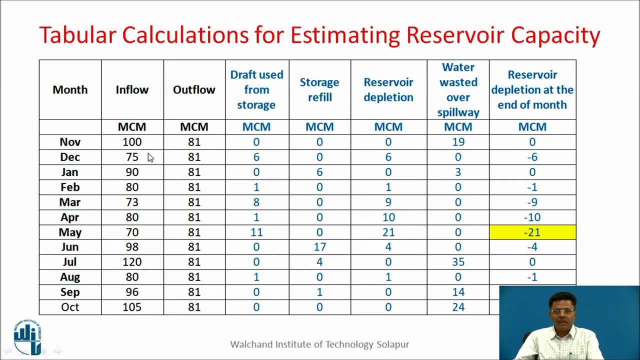 in every month to generate 7360 kilowatt continuously. now here inflow as it is given in our question: November, December, January, February, March, April- you find it is varying. and outflow we are assuming constant for generating 7360 kilobytes of energy. that's why it is. 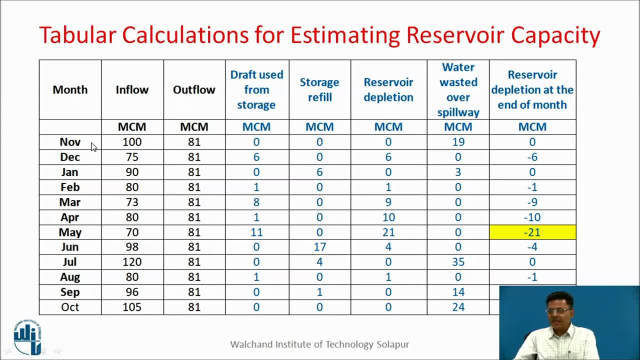 same now as reservoir is full at start of November. in month of November inflow received is 100 whereas outflow used is 81. so naturally excess of this water, excess over 81, will be wasted over spillway. again, by end of November the reservoir is full. 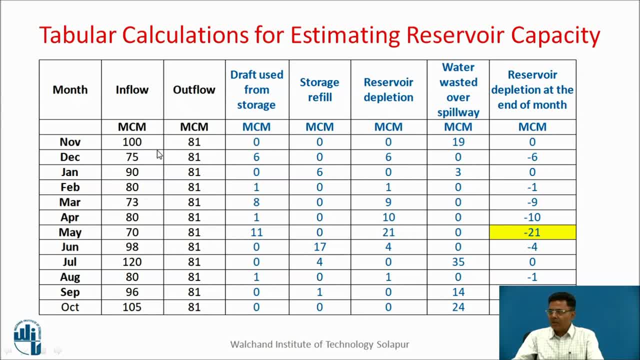 when you come to December, inflow is 75 and offflow is 81. it means off flows more. So we will have to take 6 million m3 of water from storage. That is why draft used from storage is 6 and by end of December 6 million m3 will be the. 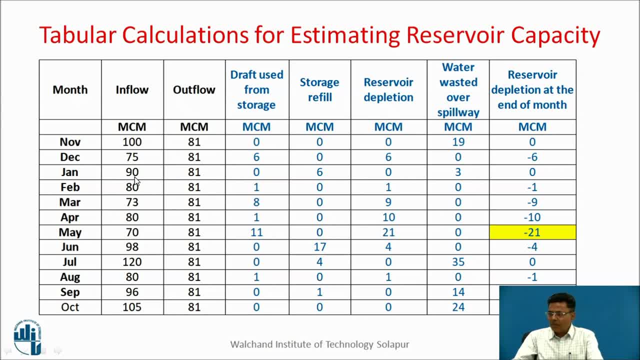 depletion in reservoir In month of January we find that inflow is 90, outflow is 81. It means 9 million m3 excess water has come. So this excess water will be used for refill first. So 6 million m3 will be refilled. 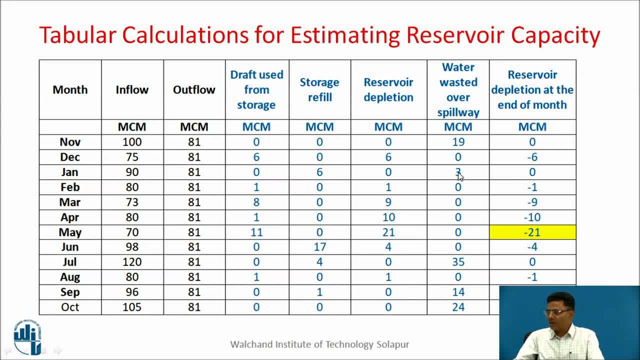 That is why the 3 million m3 of water will be wasted over the spillway. Here we come to February. inflow is 80, outflow is 81. So draft used from storage is 1, reservoir depletion is 1.. 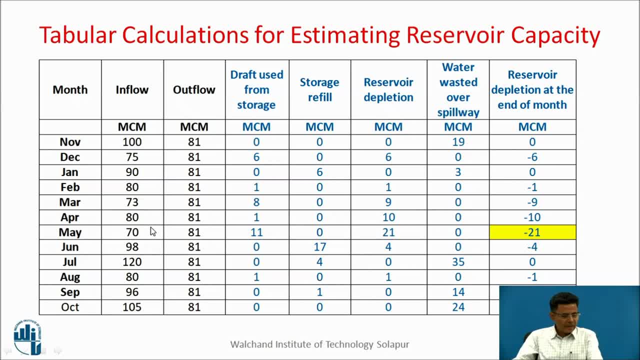 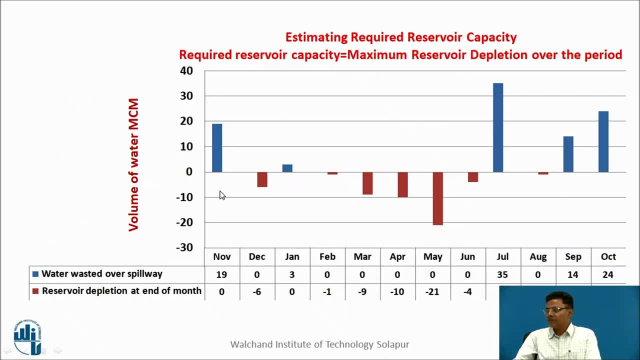 So we proceed with such a situation, Such calculations, and ultimately we come to see that maximum depletion observed is minus 21.. It means where there is excess, you can imagine that this is reservoir full condition indicated by horizontal. Then when you come here in month of January, the spill is 19.. 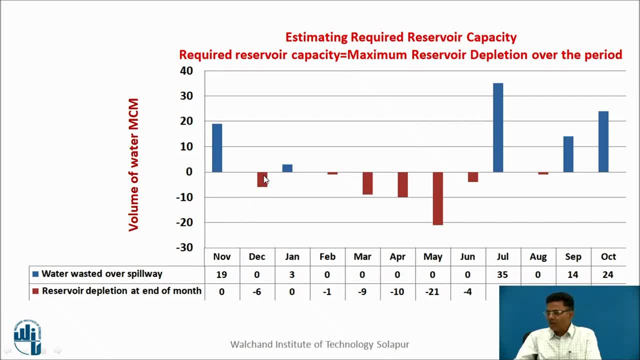 But in month of December we are using 6 million m3 from storage. In March we are using 6 million m3. We are using 9 million m3 from storage And maximum we are using 21 million m3 in month of May. 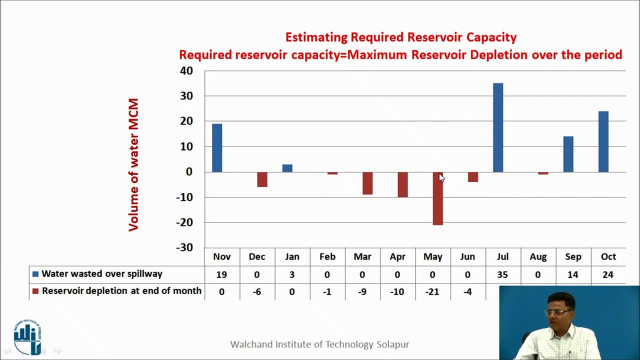 So over a period of time, we find that the maximum depletion from reservoir observed is 21 million m3.. So if we provide 21 million m3 as storage, then every demand over a period of time will be satisfied. So this is the analytical method. 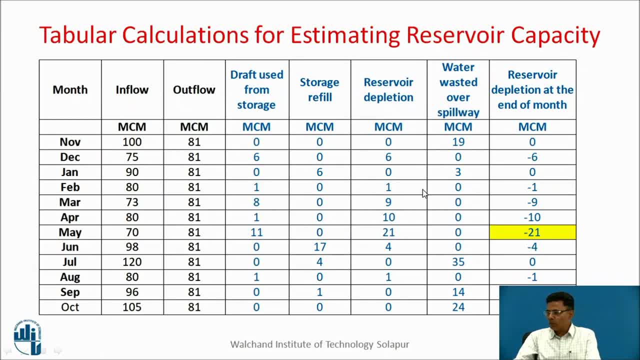 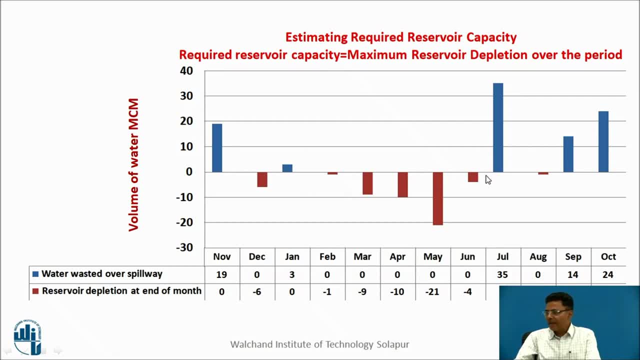 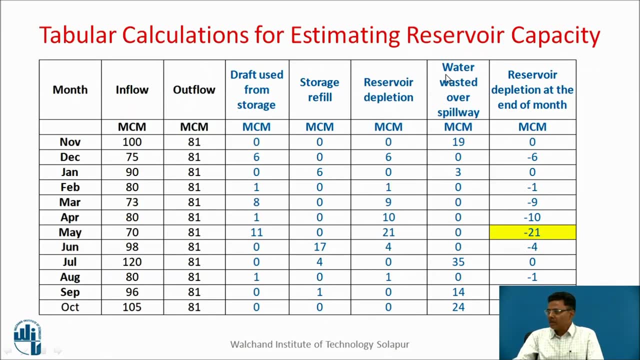 And the answers are shown by using this particular graph here, And the volume of water which is discharged over a spillway is shown in this way, in particular months or so. So if you come here, you will find these are the values of water wasted over spillway. 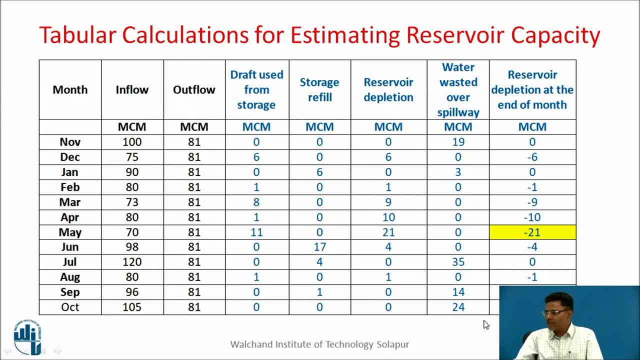 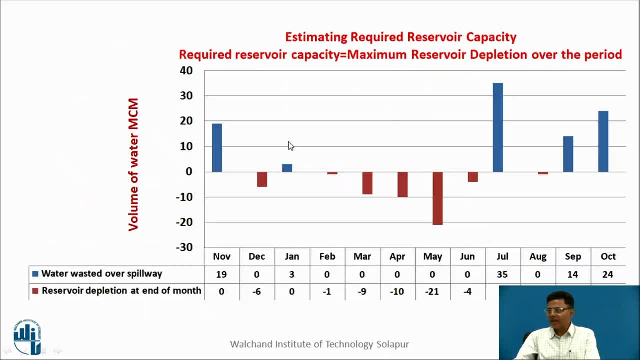 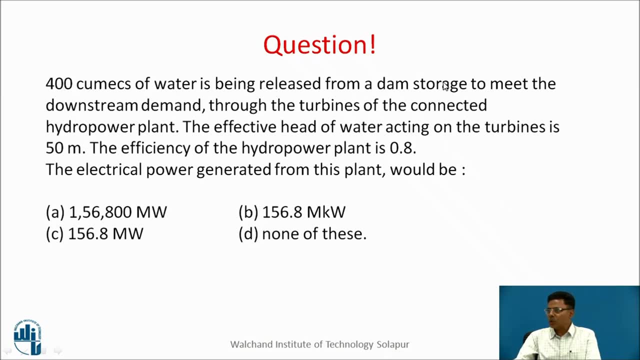 And these are the values of reservoir depletion. When you find some of all these, you will be getting water wasted over spillway And maximum reservoir depletion will be the required reservoir capacity. So last question: 400 cubic of water is being released from a dam storage to meet the downstream demand.